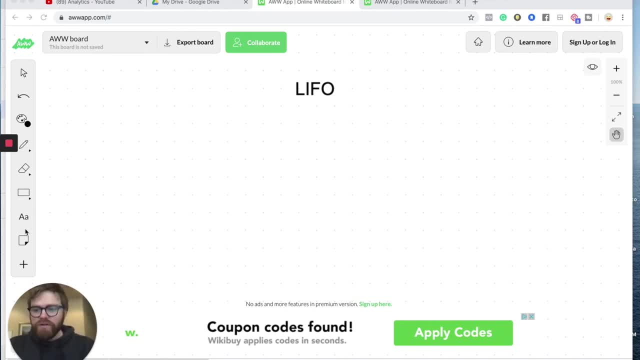 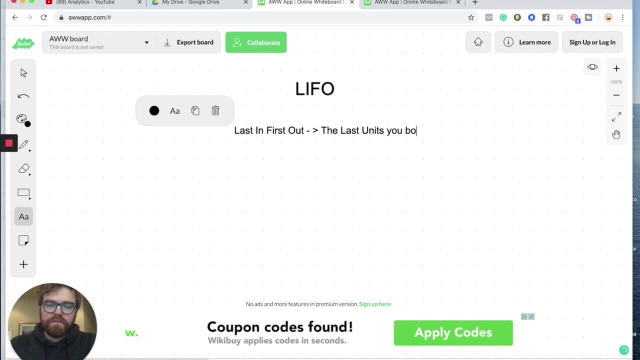 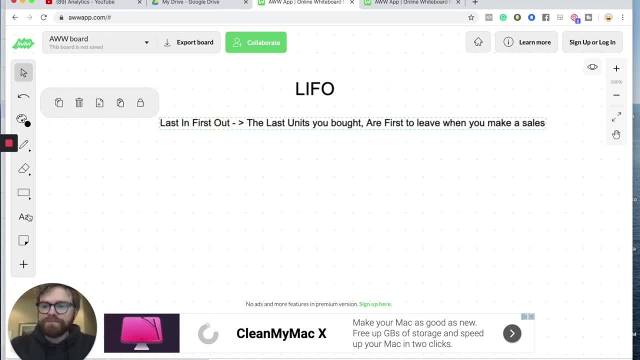 bit All right. So that's essentially what LIFO really means. In the FIFO video, if you watched that, I made an example about groceries. When you go and try to make a sauce, you should take the oldest tomatoes out first to make the sauce. And that's FIFO, With LIFO: last in, first out again. 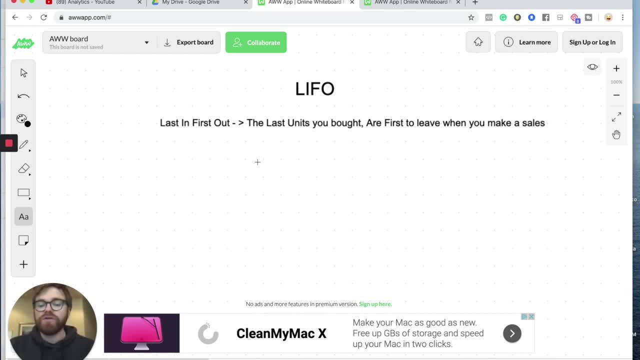 it's the last thing that you purchased you should use first. We can use that same example with the tomato sauce. If you go to the store and you're buying tomatoes to make a sauce, you're going to want to use the tomatoes that you already had in your fridge first to make the sauce, so they don't. 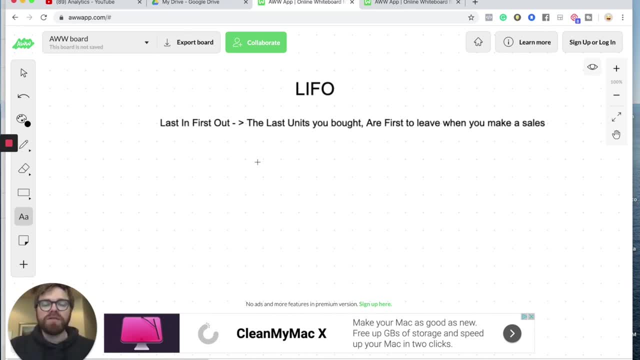 go bad. But let's say you're going to go to the fridge again. you bought some tomatoes, you're putting them away and you see an old tomato. You're going to want to use the tomatoes that you already had in there. But that tomato it's bad, It's gone really bad. You don't want to use it. 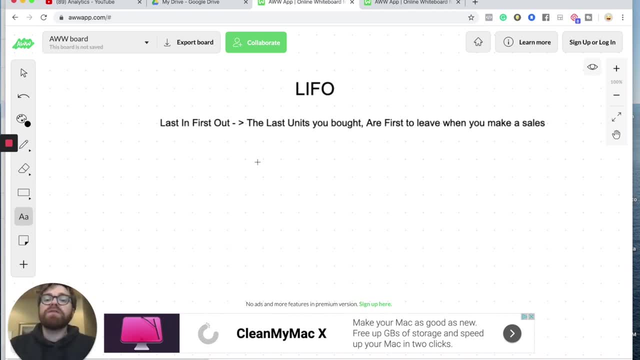 anymore. So in this situation you would take the most recent tomatoes you bought to make the sauce. Same deal here. You take the most recent inventory, or you can say last inventory, the last ones you bought to use first for the sale. That's what LIFO is, And there's some. 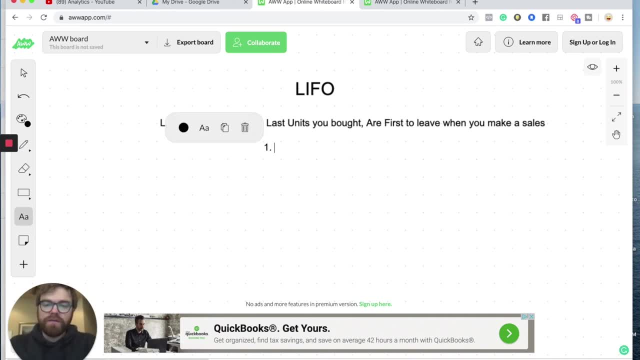 rules about LIFO here that you should know. So the first rule here is: we'll go back to the LIFO here. So the first rule here is: we'll go back to the LIFO here. So the first rule here is: we'll go back. 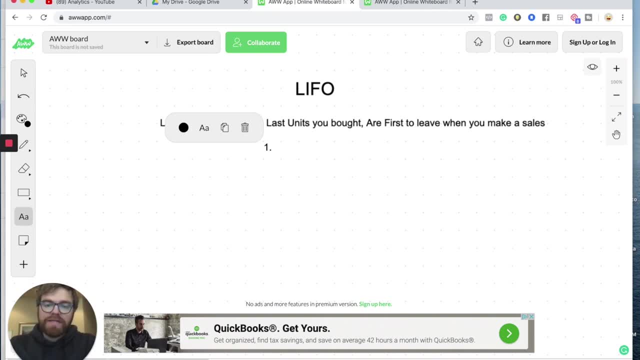 over it. Your last or most recent purchases go to cost of goods sold. That means your older purchases go to ending inventory. That's what's left over. So, in a period of rising prices, what's going to happen is your cost of goods sold under LIFO. 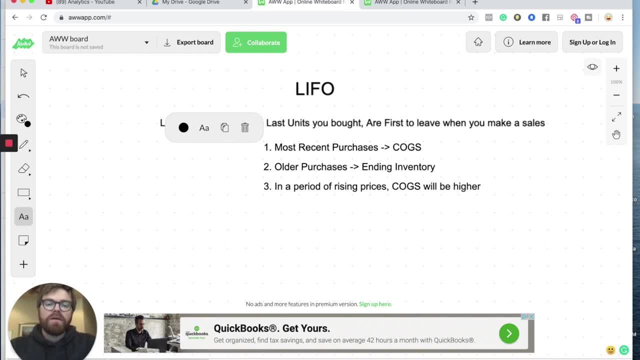 will be higher. Now think about it. Your most recent purchases- you took the last purchases- usually are more costly, And that goes to cost of goods sold first, So your cost of goods sold will be high. In that respect, though, ending inventory will be low. It's left with a lower value, So it 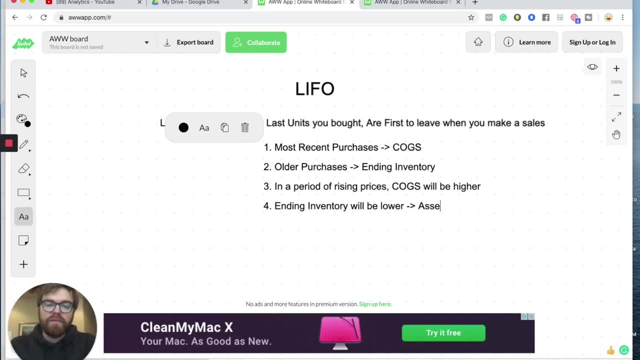 lowers your assets. right Inventory goes on your balance sheet. It lowers your assets. Lastly, if your cost of goods sold is high, that means your income is low, But also your taxes are low. So those are some basic characteristics of LIFO. Let's jump over to. 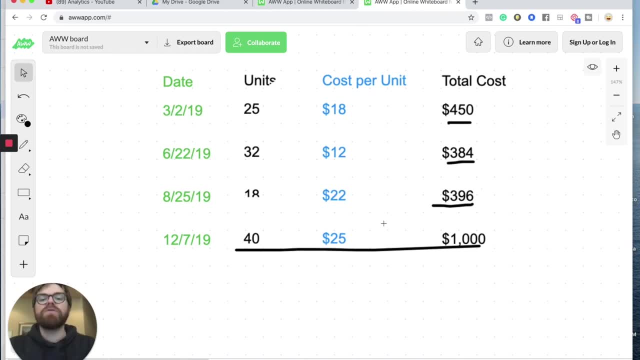 an example. So over here I'm using the same numbers as in the FIFO video just to show you how LIFO works. So let me get my pen out And yeah, that should be fine. So let's say that you sell and we'll use a different number here. We sold 100 units. You sold 100 units. How do we? 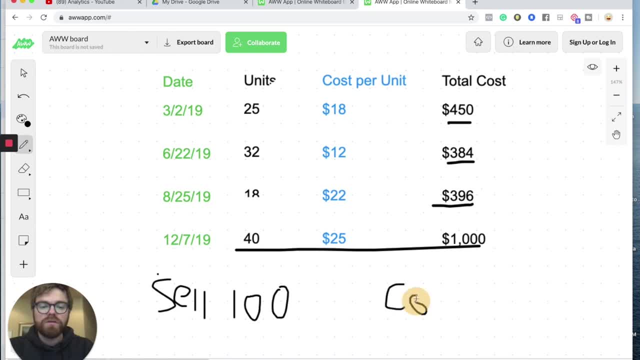 account for. We're looking for cost of goods sold. We're looking for cost of goods sold. We're looking for cost of goods sold and ending inventory. Okay, those are the two things we're looking for. So let's go ahead and think about it. We sold 100, and we know with LIFO to get our cost of goods. 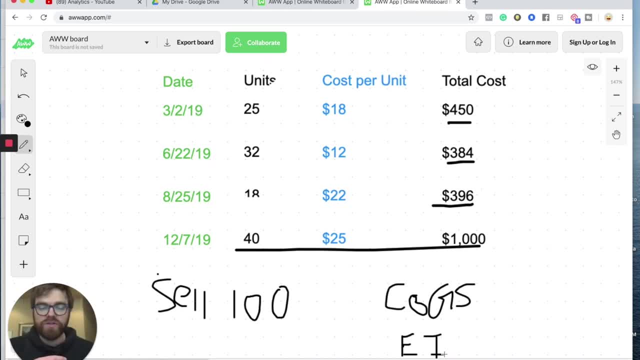 sold. we take our most recent inventory out first to assign to it. So our most recent one was right here on December 7th. We sold 100. So let's go ahead and take out all of this 40 here. Now we know it's going to be $1,000 so far for that. Just to let you know real quick your units. 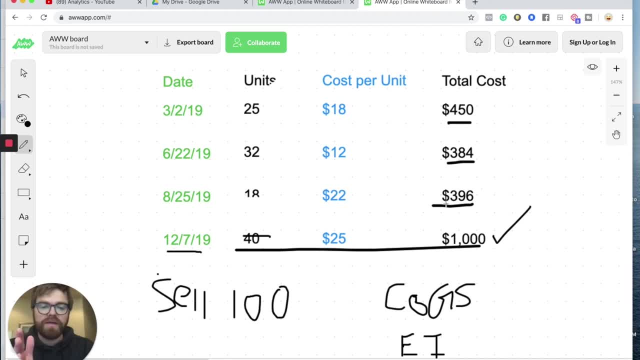 are over here: your cost per unit and the total cost. I just multiplied these together just to let you know. That's how those numbers came about. But back to the example. So we sold 100, and we took out 40 from this batch. We know this batch is 18.. We'll take out all of that, So 396.. We started with.